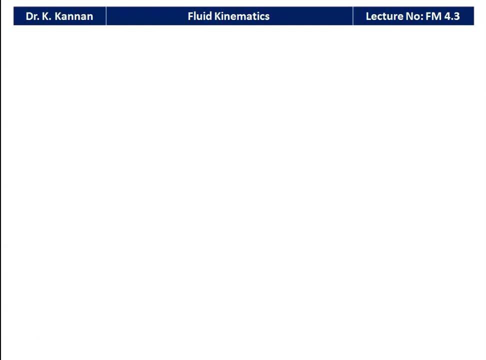 fourth chapter, third lecture. The topic what we are going to discuss is fluid kinematics. So, in the fluid kinematics, we will be discussing about velocity and acceleration, circulation and vorticity, and velocity potential function. 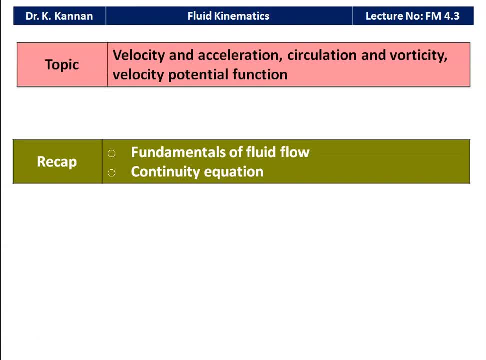 So, in the earlier lecture, in the fourth chapter, we studied about the fundamentals of fluid flow. We classified the flow into different types, steady flow, unsteady flow, uniform flow, non-uniform flow, compressible flow, incompressible flow, rotational flow, non-uniform flow, non-uniform flow. 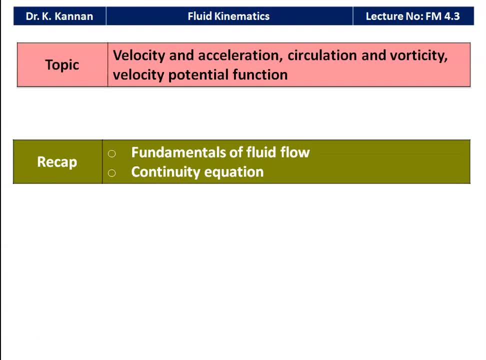 Irrotational flow, one-dimensional, two-dimensional, three-dimensional flow. 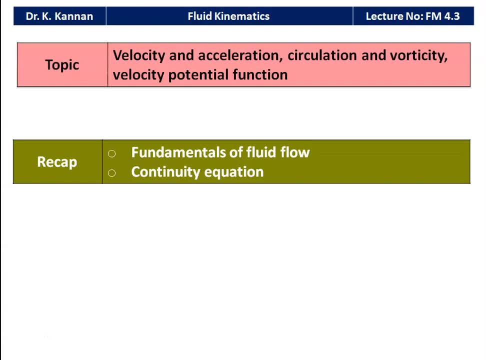 So, there are different types of fluid flow. And we derived the continuity equation. So, based on the mass conservation principle, we derived the continuity equation which is 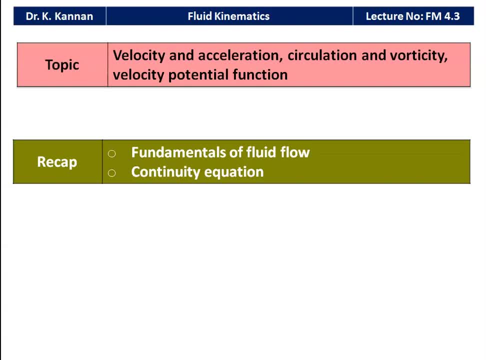 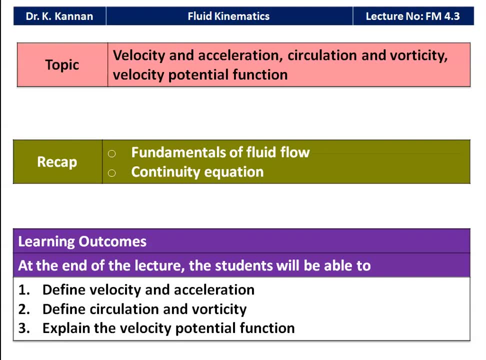 applicable for the fluid flow, fluid mechanics subject. And the learning outcome for this lecture, so at the end of the lecture, the student will be able to define velocity and acceleration. 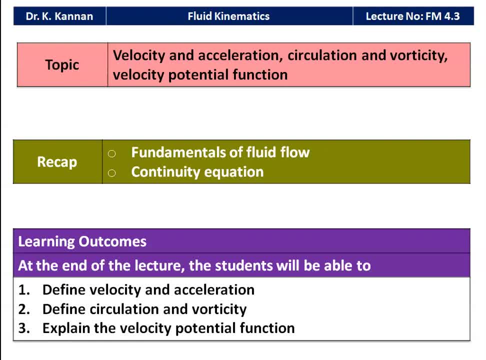 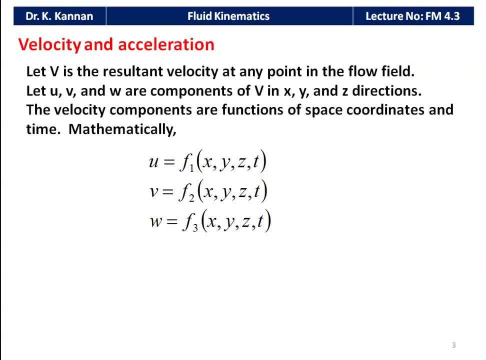 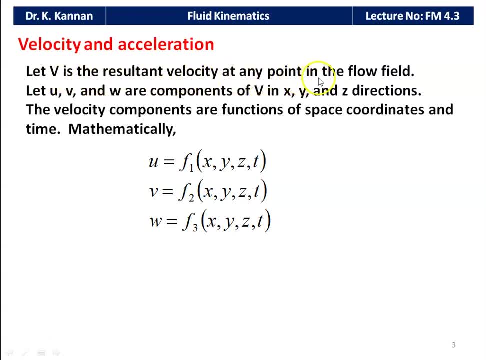 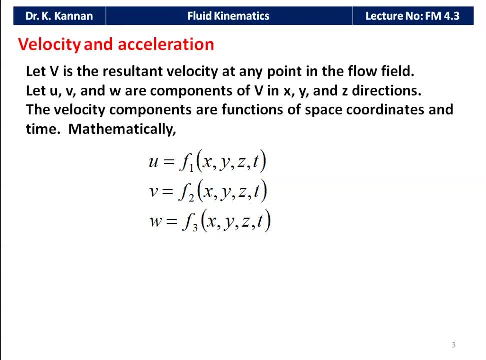 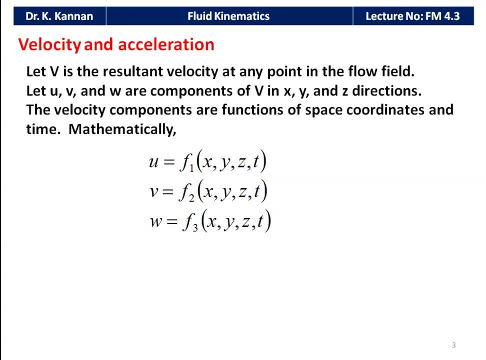 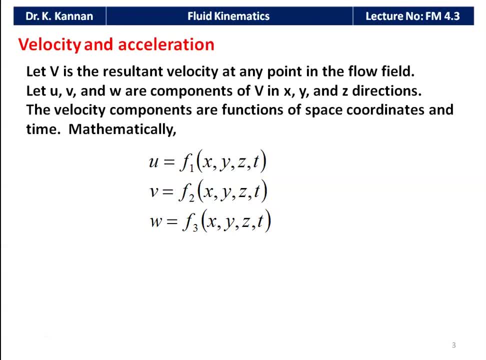 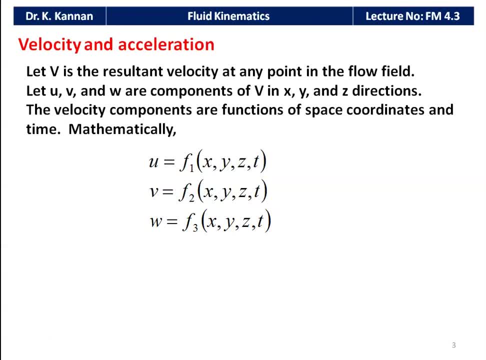 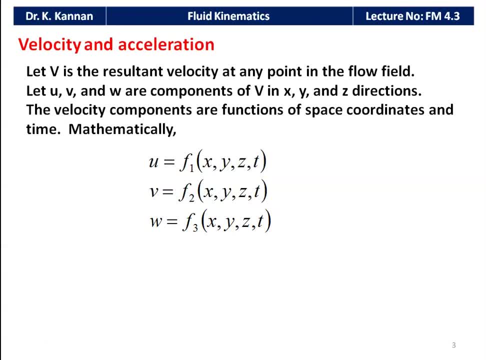 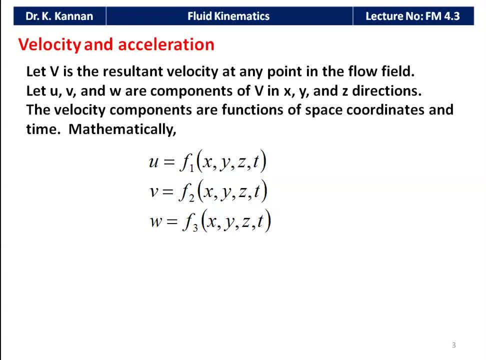 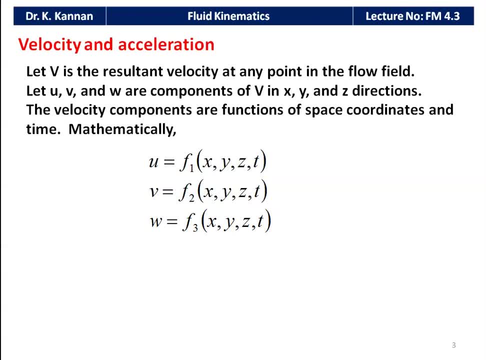 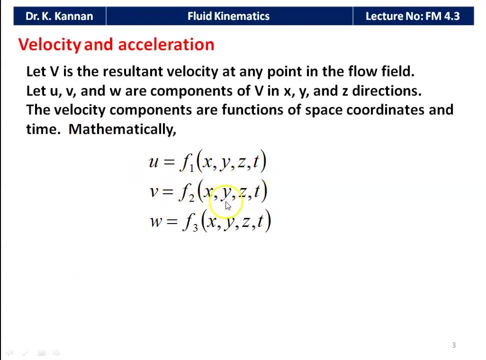 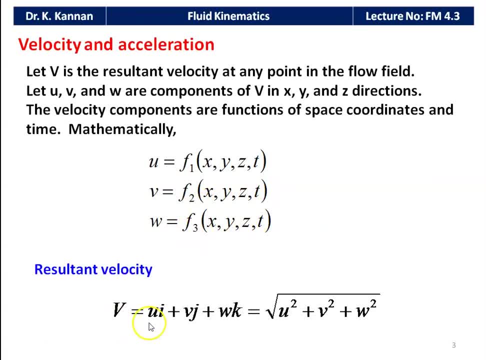 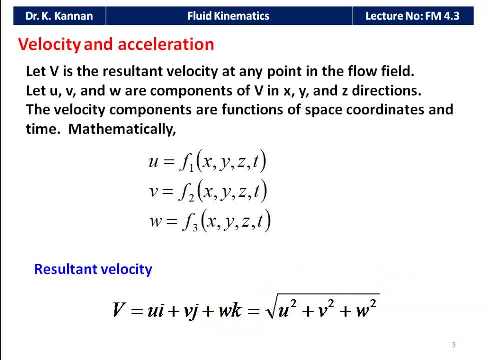 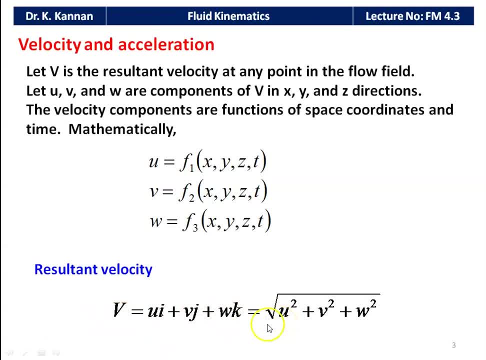 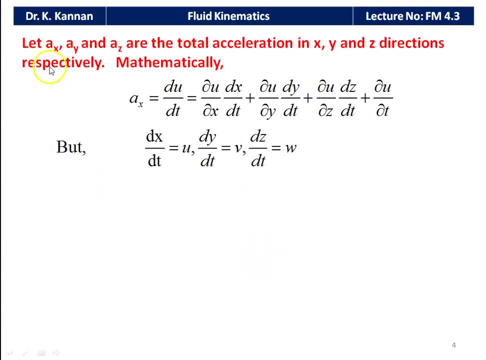 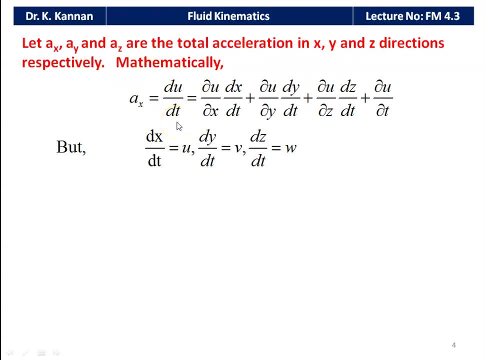 systematically A x equal to d u by d t. So, we know u is a function of x, y, z and t and differentiating dou u by dou x A d x by d t plus dou u by dou y d y by d t plus dou u by dou z d z by d t plus dou u by dou t. So, velocity acceleration u is a function of x, y, z x, 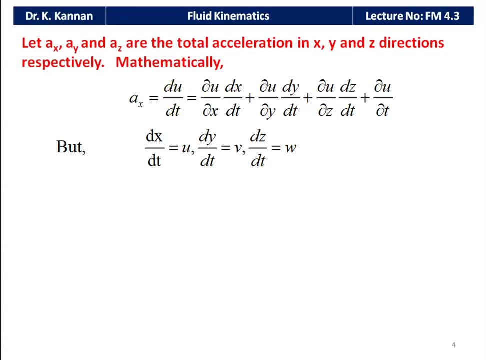 y, z and t that we have seen in the previous slide. Now, here the change in the length in the x direction with respect to time is called as u velocity. Similarly, change in the y direction length in the y direction with respect to time is v velocity and d z by d t equal to w. 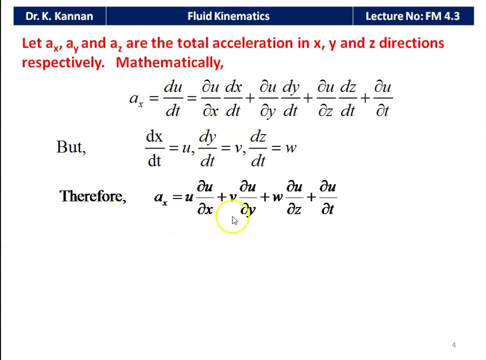 So, substituting A x equal to u into dou u by dou x plus v into dou u by dou y plus w into dou u by dou z plus dou u by dou t and this equation also you have to remember. 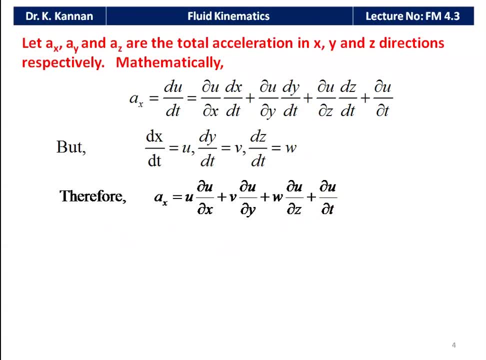 There are acceleration in the x direction u into dou u by dou x plus v into dou u by dou y and w into dou u by dou z plus dou u by dou t and similarly, we can write in the y and z direction. So, A y equal to u into dou v by dou x plus v into dou v by dou y plus w into dou v by dou z plus dou v by dou t and A z equal to u into dou w by dou x plus v into dou w by dou y and w into dou w by dou z plus dou w by dou t and the three equations you have to remember. 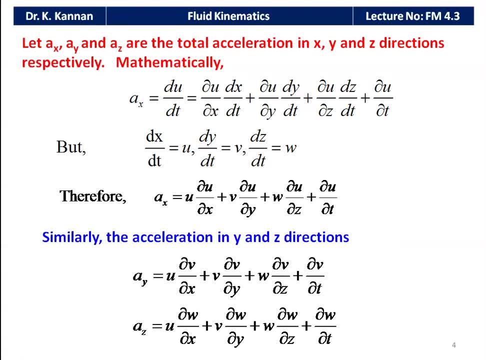 So, look at the logic. So, if you understand the logic, then you can easily remember. So, in all the four terms, first three terms, you have u v w in the same sequence. 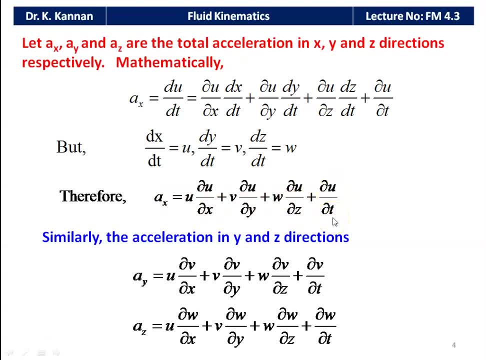 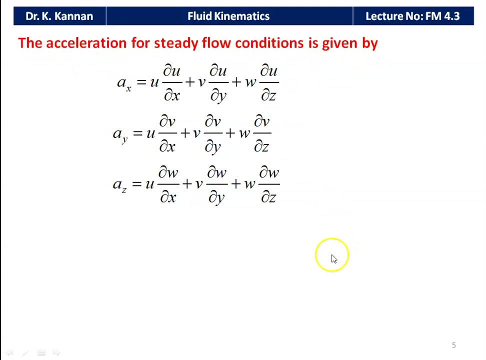 Last term, the velocity is differentiated with respect to time. So, dou u by dou t, dou v by dou t, dou w by dou t and in the three term, you have u v w, here dou u by dou x, dou u by dou z. So, u is the velocity in the x direction. So, differentiating with respect to x, y and z direction. Similarly, here v is the velocity in the y direction. So, dou v by dou x plus dou v by dou y plus dou v by dou z and the w is the velocity in the z direction. So, dou w by dou x plus dou w by dou y plus dou w by dou z. So, if you understand the logic of writing the expression, then you can easily remember. And the acceleration for a steady flow condition, for steady flow condition, there is no change in the velocity with respect to time. So, the time dependent parameter is deleted. So, a x equal to u into dou u by dou x plus v into dou u by dou y plus w into dou u by dou z. a y equal to u into dou v by dou x plus v into dou v by dou y plus w into dou v by dou z. And a z equal to u into dou w by dou x plus v into dou w by dou y plus w into dou w by dou z. 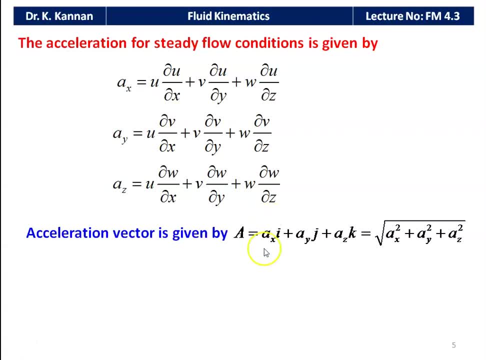 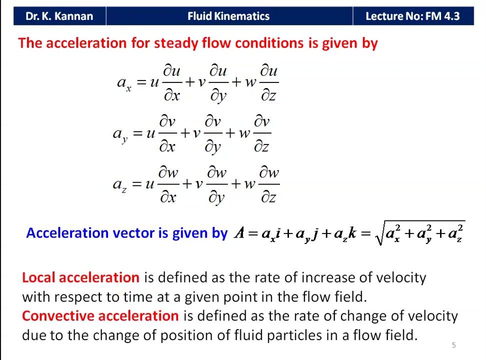 Then the acceleration. Acceleration a is calculated by a x i plus a y j plus a z k. So, it is square root of a x square plus a y square plus a z square. And the resultant acceleration, this equation also you have to remember. So, this is also useful for solving problem in the flow field. Then the acceleration there are two types. One is local acceleration and another one is is convective acceleration. So, local acceleration is defined as the rate of increase of velocity with respect to time at a given point in the flow field. So, rate of, you may look at the definition rate of the increase of velocity with respect to time at a given point in the flow field that is what local acceleration. Convective acceleration is rate of change of velocity due to the change in position of the fluid particle in the flow field. So, with respect to time is local acceleration, with respect to position the derivative, the change of velocity with respect to position in the flow field it is convective acceleration. 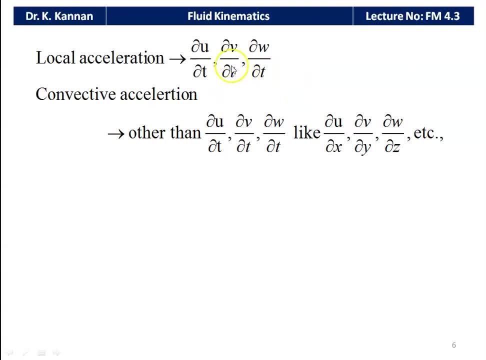 And from the definition of the point, so the term dou u by dou t dou v by dou t and dou w by dou t they are the local acceleration and the convective acceleration are other than dou u by dou t dou v by dou t and dou w dou t like dou u by dou x dou v by dou y dou w by dou z etcetera. 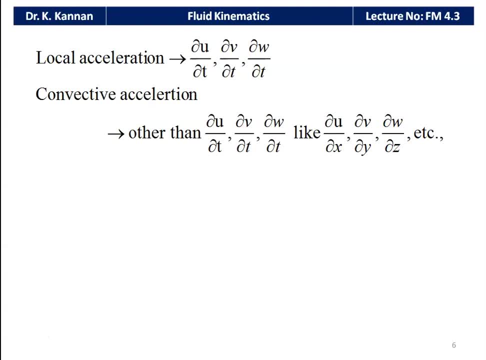 So, there are many terms convective acceleration. So, the first the time dependent parameter they are the local acceleration. And the next two parameter is circulation and the vorticity. So, fluid particle and can undergo the following four types of displacement. So, when the fluid is flowing 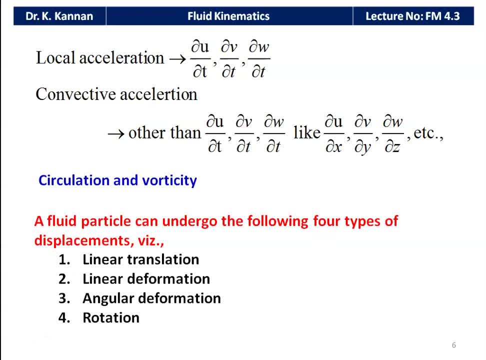 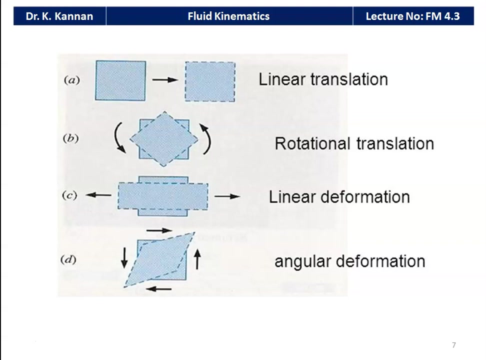 through a pipeline or when the fluid is flowing through a open channel the fluid is flowing but there are four different types of displacements. So, the fluid particle is moving from one place to another place there are four different possible movements are possible. One is linear translation, linear deformation, angular deformation and rotation. And look at the diagram you can understand. So, A is linear translation. So, the fluid particle without changing the shape it is moving. 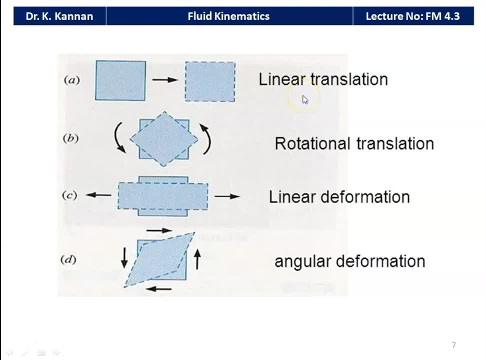 In a linear direction that is what linear translation. So, fluid particle moving in a 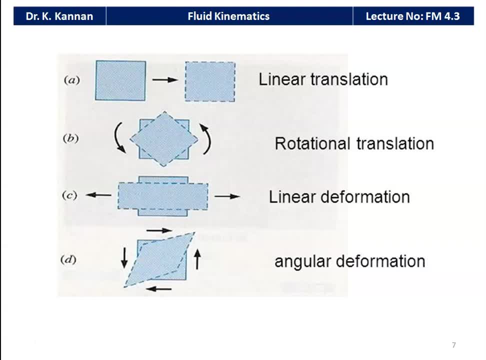 open channel you just think of a fluid particle. So, when there is a fluid particle that is moving in the linear direction. Then rotation when the fluid particles are rotating about the center mass center that is called as rotational translation it is rotating about the center 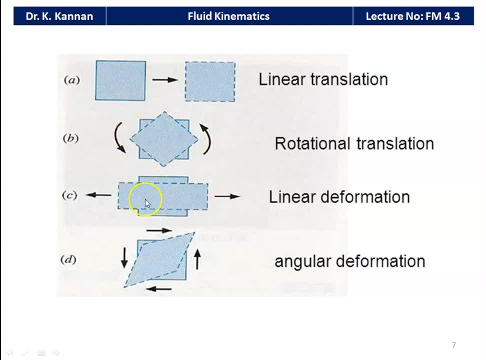 in the anticlockwise direction. And linear deformation. So, look at the dottolab. 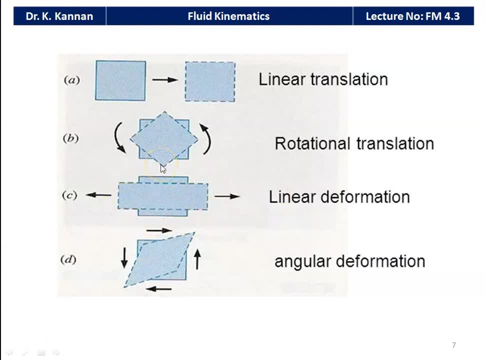 Dottolab. So, the shape is changing shape of the fluid particle is changing that is what called as linear deformation. Then angular deformation. So, the when the fluid particle subjected to 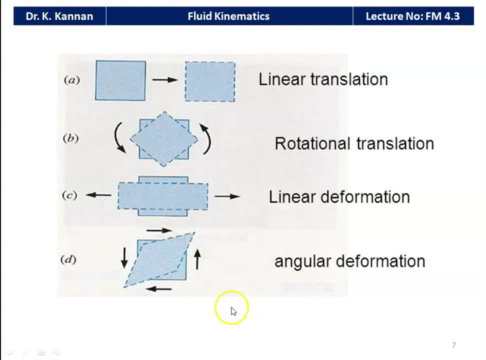 force like this it is it will give the angular deformation. So, the fluid particle when this is flowing in a flow field maybe in a closed pipeline or in a open channel open channel the four different basic movement of the fluid. Dottolab. 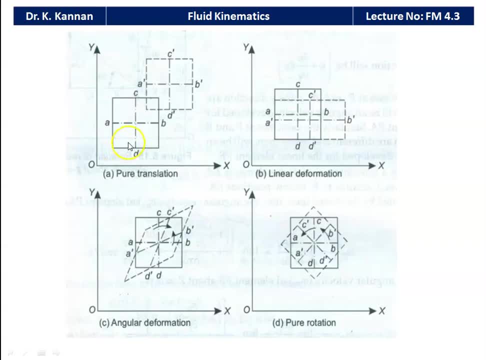 And in other words then to be able to move it is possible. Now, the you can understand they better fuel translation. So, it is moving in a linear direction a b c d is the center point and a dash b dash e dash d dash d dash is the next level. 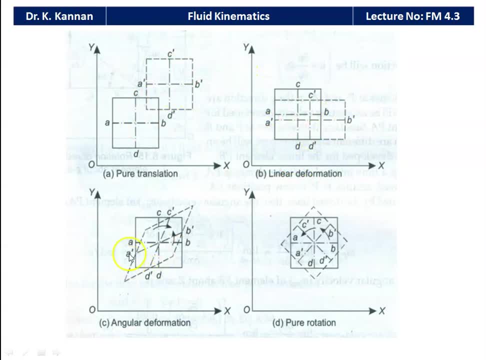 Then here linear deformation the change in the shape this is angular deformation and 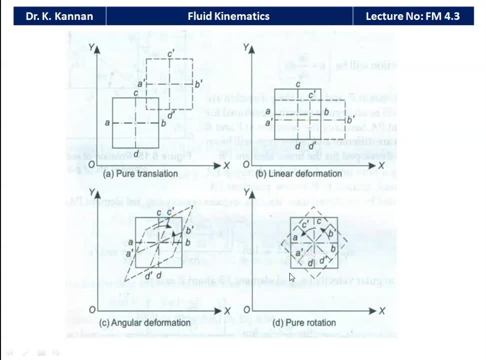 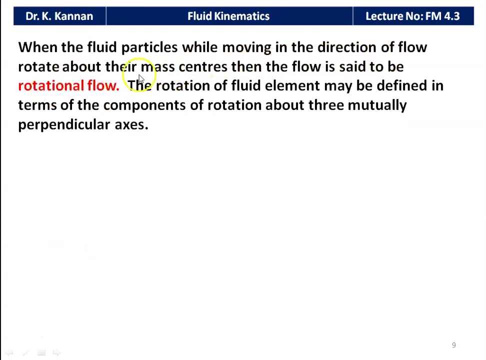 this is rotation. So, it is only a single flow fluid particles right. So, you have to look at that the microscopic level. So, when you understand the behavior of the fluid particle, single fluid particle then it is easy to understand the behavior of the entire fluid which is flowing through a pipeline or a open channel. Then when the fluid particle while moving in a direction of flow rotate about the mass center then the flow is said to be rotational flow. When the fluid particles while moving in the direction of flow rotate about the 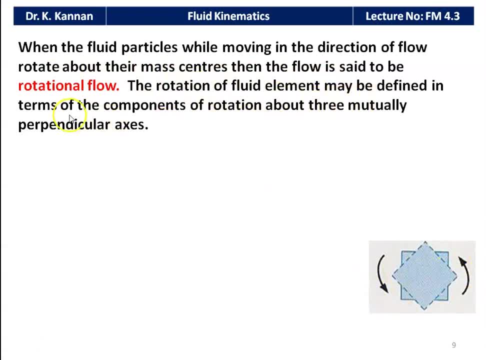 flow. The rotational fluid element may be defined as in terms of components of rotation 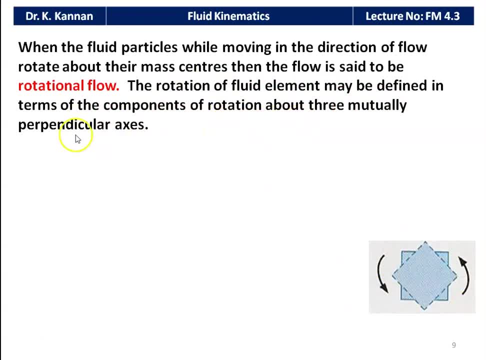 about the three mutually perpendicular axis. So, everything, so if it is a rotation physically 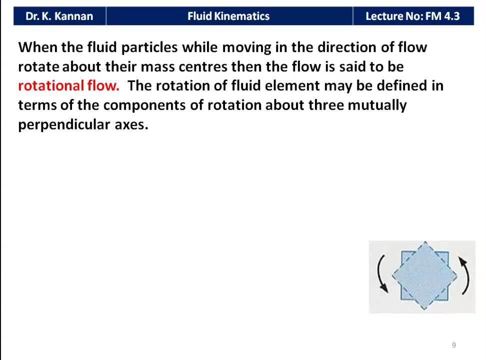 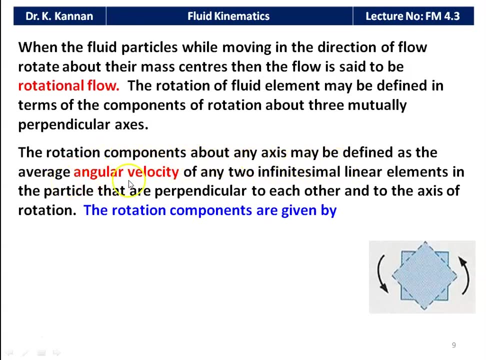 we can visualize the rotational rotation of the fluid particle, but we have to represent the movement mathematically then only it is easy for analysis. So, we have to represent the rotation mathematically. Rotation of rotation components about any axis may be defined as the angular velocity. So, this is the radial velocity in this case the angular velocity given for rotation of any two diameters any two infinite decimal linear element that is perpendicular to each other and the axis of rotation. Rotational components are given by Omega x rotation about the X axis Omega y rotation about the y axis Omega z rotation about the Z axis. So, look at the component rotational component 1 by 2, dou W by dou y minus dou v by dou z. Omega y 1 by douётся or miss the siglo power've it come down to 1 minus 1 minus take it 1 by 2. But, if this is theot significative relation that, this is the because the 다음에 So, this is a Dr PrayEP . This is the theoretical requirement. The former one is liquid Host function associated with the Chron��고 of the angle it will go on to pH level when shown It is a nice, very direct interpretation. There are nod Pop is notください. So, we know what 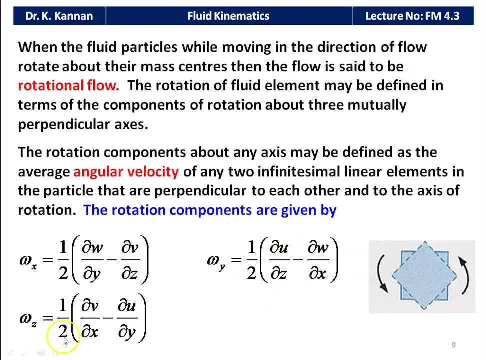 to dou u by dou z minus dou w by dou x, omega z 1 by 2 dou v by dou x minus dou u by dou y. 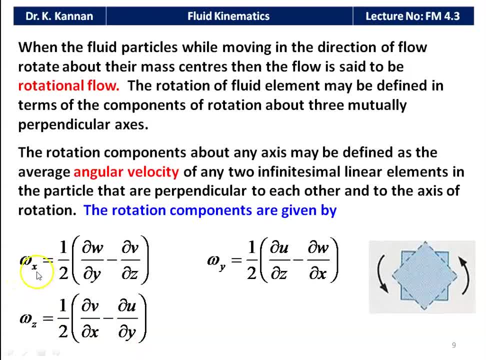 Then again how to remember this equation? So, omega x, so it is rotating about the x axis, x direction, x point in the x axis. So, look at here the other two directions are other two components are available. So, dou w velocity in the z direction and differentiating with respect to y direction, dou w by dou y minus dou v velocity in the y direction divided by z direction. So, dou v by dou z, then only the fluid particle will rotate. Then similarly dou equal to, so y is the y direction, so look at the components here, the parameter here, the other two directions, dou u by dou z minus dou w by dou x, omega z, similarly it is z direction, so there will not be z and the dou v will not exist, dou v will not exist and then again, dou w by dou z, dou z will not exist. 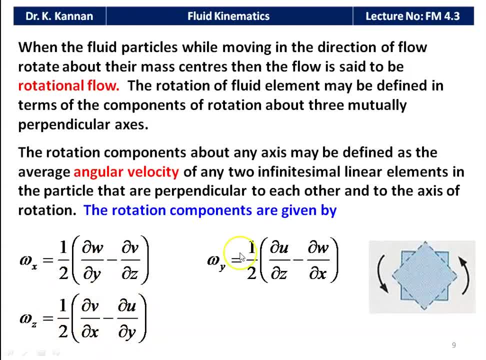 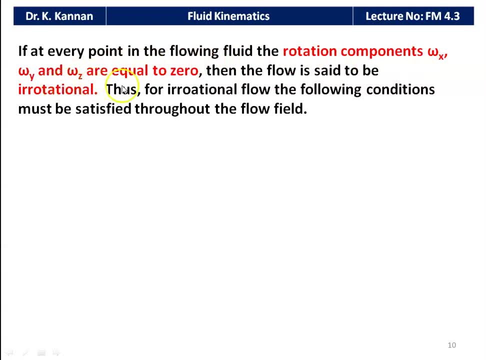 どう y by book in the foisasty formulae look at the parameter here, the other two directions, do you, by Damascus by Z minus dou w by do yx, omega z similarly, it is z direction ocho there won't be z and the do. term. So, dou v by dou x minus dou u by dou x. So, this is what? This you have to, again you have to understand the logic of writing the expression, then it is easy for you to remember. If at every point in the flow field, the rotational component omega x, omega y and omega z are 0, then the flow is said to be irrotational. So, that is for irrotational flow, the following condition must be satisfied throughout the flow field. And this is the rotational component. When omega s, x, omega y, omega z, they are 0, then the equation will be like this. Dou w by dou y equal to dou v by dou z from the first expression. Dou u by dou z equal to dou w by dou x from the second expression. And dou v by dou z, dou x equal to dou u by dou y. So, these are all the conditions for irrotational flow. 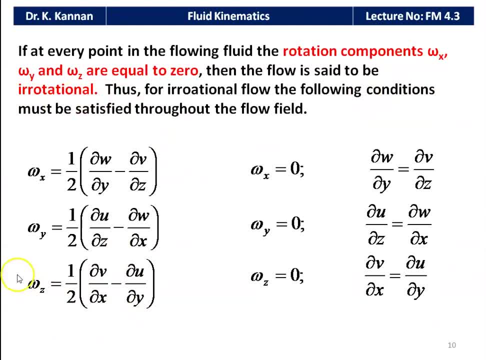 And these are all the conditions, equations for rotational flow. So, if it is rotational flow, we have to calculate. 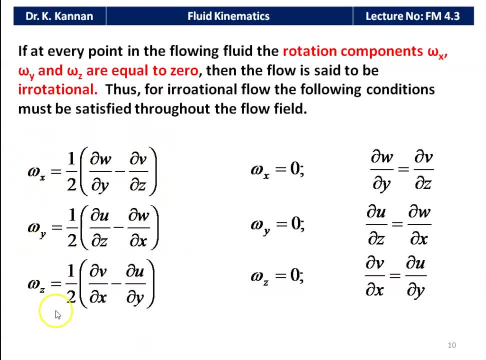 We have to calculate omega x equal to omega x, omega y and omega z. If it is irrotational 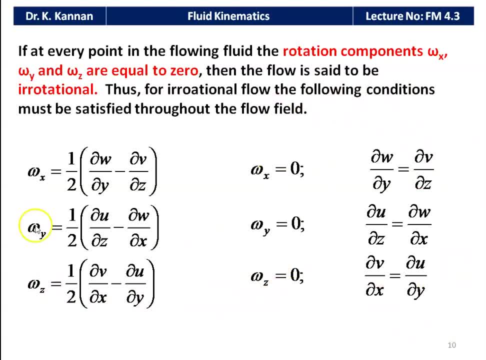 flow, and this is the condition to be satisfied. And if we define the circulation, the flow 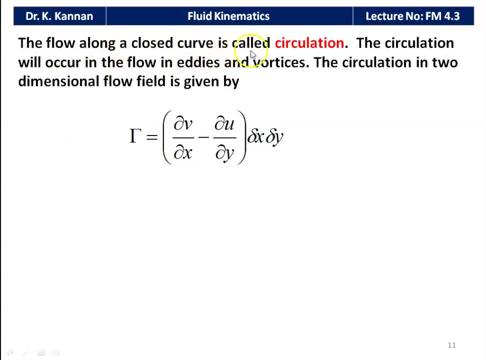 along the closed curve, the flow along the closed curve is called a circulation. The circulation will occur in the flow eddies and the vorticitys. So, circulatory flow, 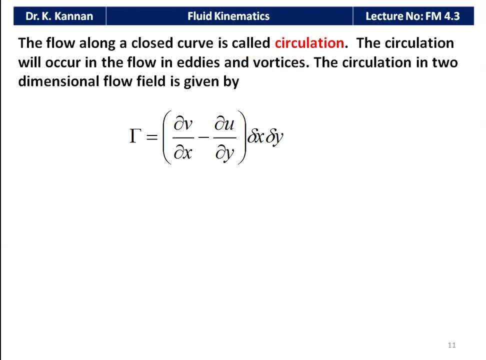 normally in the film mechanics, it is unwanted phenomena. So, we will discuss later on. So, we will discuss later about the circulation. So, the circulation will occur in the flow 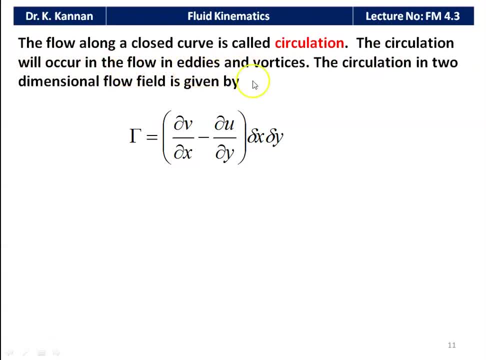 in the flow in the flow in the eddies and vorticitys. The circulation of two-dimensional flow field is defined by tau. How to pronounce it? Tau equal to dou v by dou x minus dou u by dou y delta x into delta y. And vorticity zeta. So, zeta is the Greek letter. Zeta at 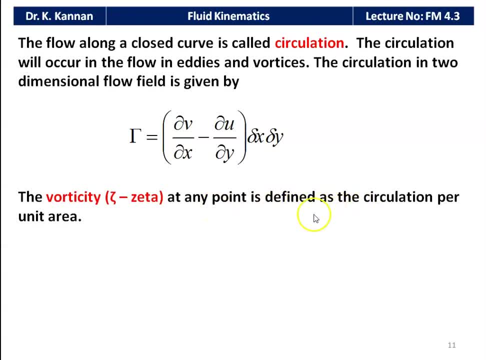 any point in the flow, flow is any point is defined as the circulation per unit area. 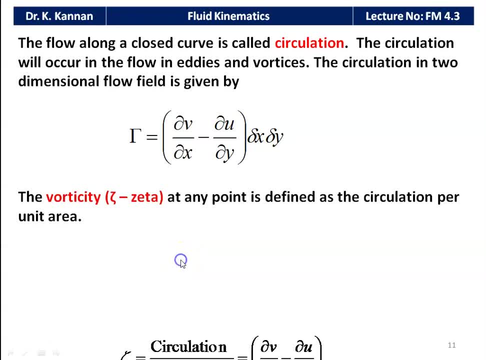 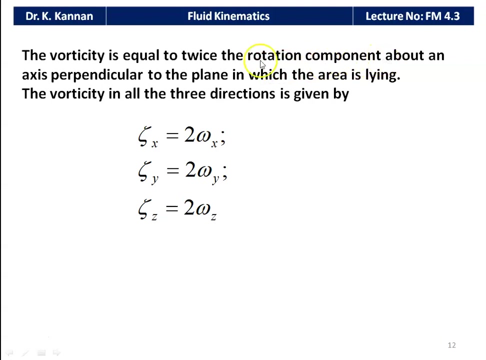 So, the circulation per unit area is the vorticity. So, defined here, zeta equal to circulation divided by the area. So, area equal to delta x into delta y. So, this tau divided by delta x delta y, this is dou v by dou x minus dou u by dou y. So, circulation, the zeta equal to 2 into omega z. What is this term? So, look at the previous slide. So, dou v by dou x equal to minus dou v dou u by dou y equal to omega z. So, the circulation equal to 2 times of omega z. Then the vorticity is equal to twice the rotation of the rotation component about an axis perpendicular to the plane in which the area is lying. The vorticity of three directions are zeta x equal to 2 omega x, zeta y equal to 2 omega y and zeta z equal to 2 omega z. So, these are all the equations that you have to remember for solving problem. 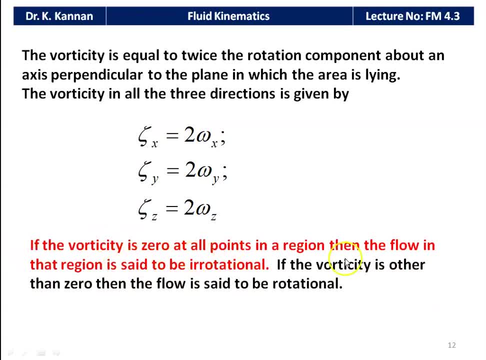 . So, if the vorticity is 0 at all point in the region, then the flow is, flow in that region should be irrotational. When zeta x equal to 0, zeta y equal to 0 and zeta z equal to 0, then the flow is called as irrotational flow. If the vorticity is other than 0, then the flow is rotational flow. So, practically the flow is rotational. Just imagine the flow of water in the river. So, it is rotating and moving. It is rotating as well as moving. So, any practical field open, open channel flow, it is rotational flow, right. So, practically the fluid flow, fluid flow is very complicated in nature, but we are, we in laboratory we are making some assumption and do our mathematical calculation in the fluid mechanics. 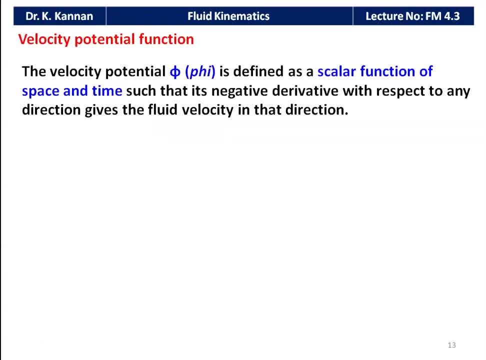 Next we define the velocity potential function. So, velocity potential function phi is defined as the, defined as a scalar functional function. . 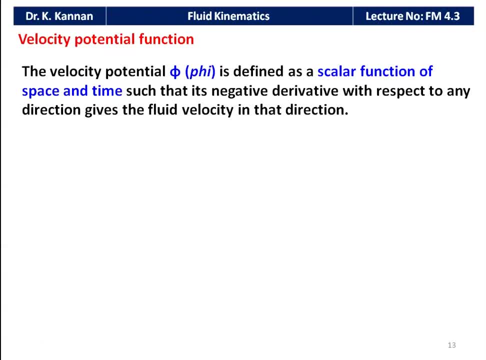 Now you can see that from the previous example, j is defined as a scalar function of space and time such that its negative derivative with respect to any direction gives the fluid velocity in that direction. So, velocity potential function is a scalar function of space and 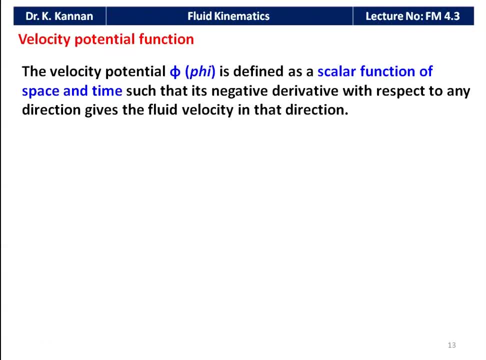 time such that its negative derivative with respect to any direction gives the fluid velocity in that direction. So, if a, if I mathematically express, it is easy to understand. So, mathematically 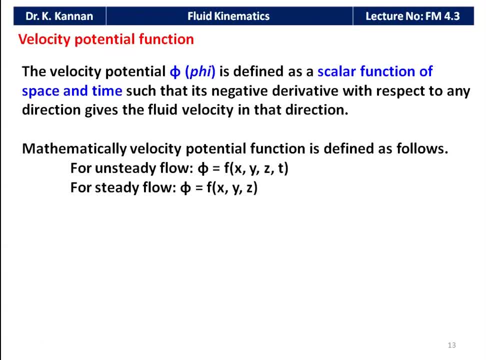 potential function is defined as for unsteady flow phi equal to a function of x, y, z and t, for steady flow phi equal to x, y, z, a function of x, y, z. And this equation is what elastic potential function. So, u equal to minus of dou phi by dou x, v equal to minus of dou phi by dou y and w equal to minus of dou phi by dou z. Now, writing this equation, you can, now you 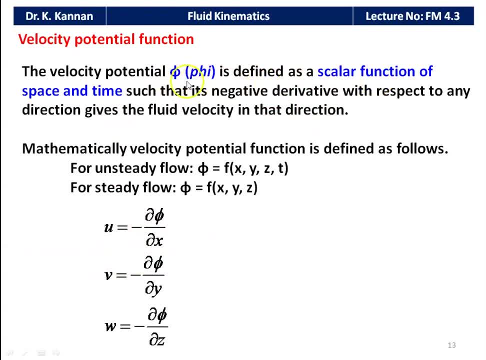 look at the definition. Velocity function phi is defined as the scalar function of space and time such that its negative derivative with respect to any direction gives the fluid velocity in that direction. So, what is negative derivative? Minus of dou phi by dou x, x direction, differentiating phi with respect to x direction that gives the velocity in that direction. 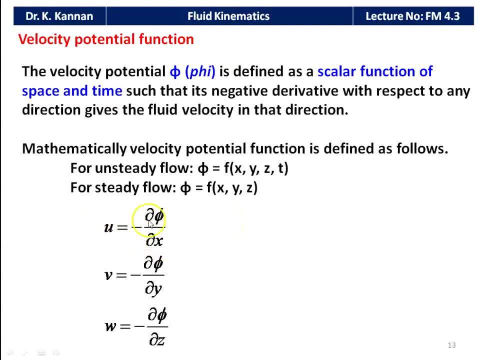 What is velocity in the x direction? u. So, u equal to minus dou phi by dou x, v equal to minus of dou phi by dou z. So, u equal to minus of dou phi by dou x, 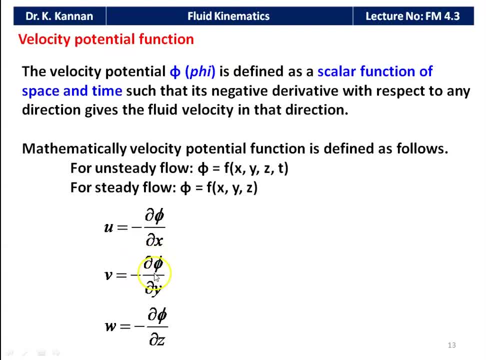 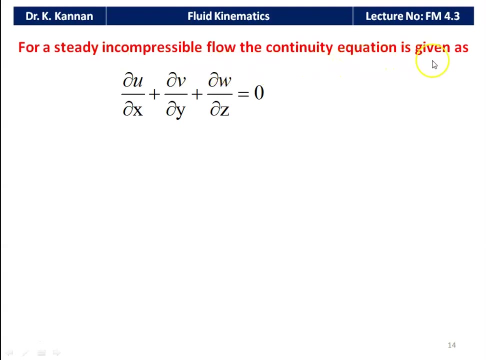 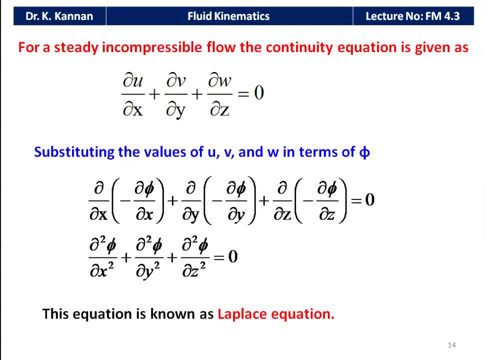 equal to 0 and this is called as Laplace equation. So, in mathematics, you will, you may be studying the second-order partial differential equation. So, this is a second-order partial differential equation for three variables and this is called as Laplace, three-dimensional Laplace equation. So, the pla and, what we saw in my lecture is in�� or note, in later lecture, we had accepted that that equation so it is the second order partial differential equation as you have seen earlier as 2 plus 2 du by delta z. So, some is Russian this, some it is also using the 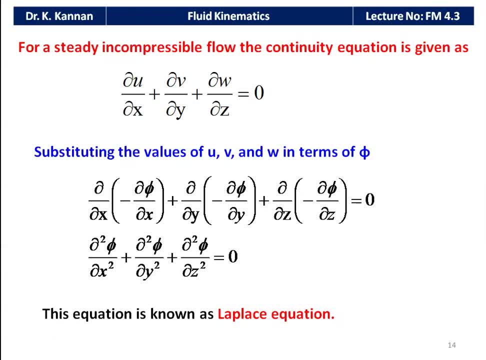 This equation is called as three-dimensional Laplace equation. For rotational flow, 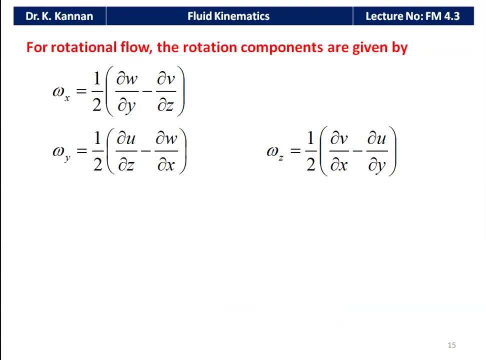 the rotational components are given by omega x equal to 1 by 2 dou w by dou y minus dou v by dou z, omega y equal to 1 by 2 dou u by dou z minus dou w by dou x and omega z equal to 1 by 2 dou v by dou x minus dou u by dou y. Now, once again we substitute the u v w in terms of phi. So, omega x equal to 1 by 2 minus dou square phi by dou y dou z plus dou square phi by dou z dou y, omega y equal to 1 by 2 minus dou square phi by dou z dou x plus dou square phi by dou x dou y and omega z equal to 1 by 2 minus dou square phi by dou x dou y plus dou square phi by dou y dou x and phi is a continuous function then. So, these are conditions. 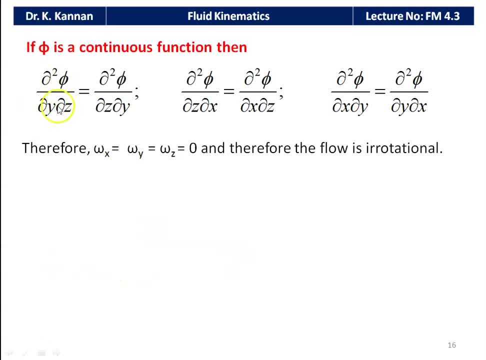 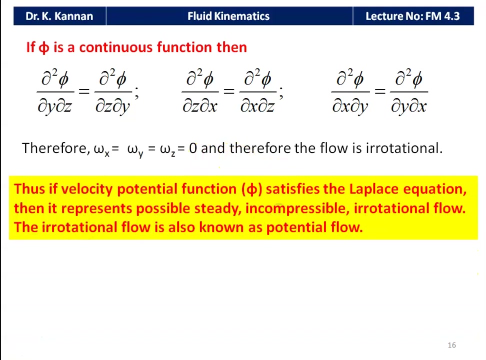 So, from here phi is a continuous function. So, we have the dou square phi by dou y dou y dou z equal to dou square phi by dou z dou y, dou square phi by dou z dou x equal to dou square phi by dou x dou y and dou square phi by dou x dou y equal to dou square phi by dou y dou x. So, therefore, omega x omega y omega z equal to 0, the flow is irrotational. So, if the velocity potential 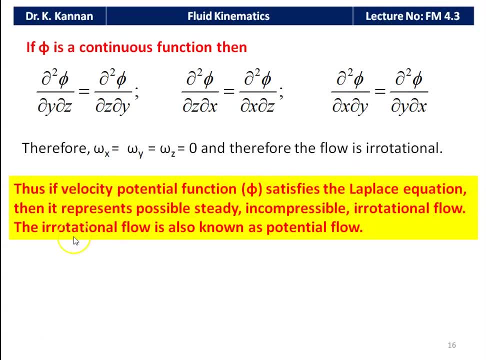 function f phi satisfy the Laplace equation, then it, it represents possible steady incompressible irrotational flow. 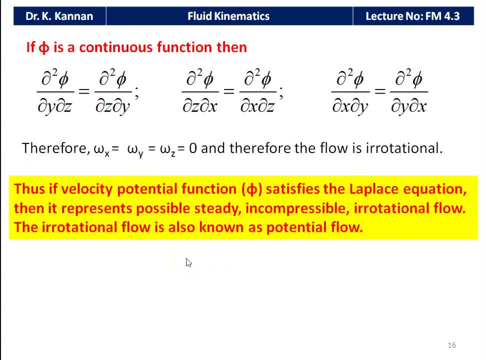 So, this conclusion you have to remember. They will give you a problem and verify whether this is steady incompressible irrotational flow. So, what is, what you have to do? We have to find out the phi terms and substitute in the Laplace equation and you have to conclude, 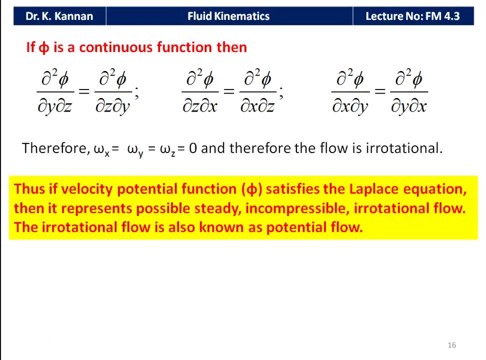 we have to find out the solution, solution should be equal to 0. When the velocity potential function satisfies, satisfies the Laplace equation, then it represent the possible steady incompressible irrotational flow. When the velocity potential function is not 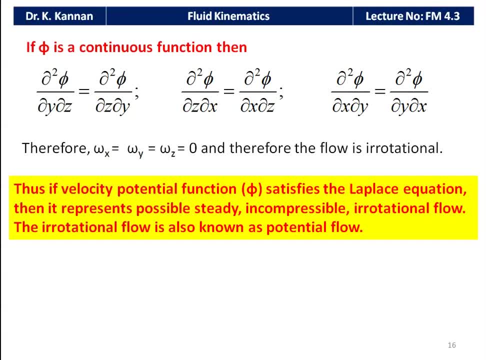 satisfying the Laplace equation, then the condition is not satisfied. So, irrotational flow, they are called as potential flow. So, remember this conclusion, the irrotational flow is called as potential flow. So, later on we will classify the flow, potential flow 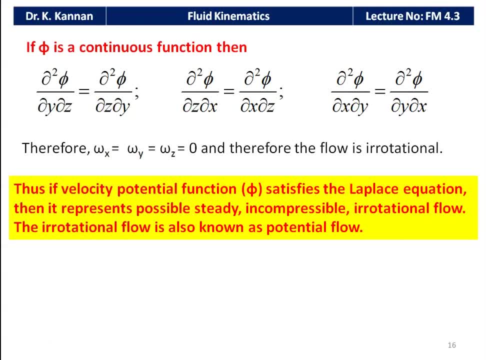 and the other type, laminar flow, turbulent flow like that, we, potential flow and another type of flow. So, the condition is when the flow is irrotational, then it is called as potential 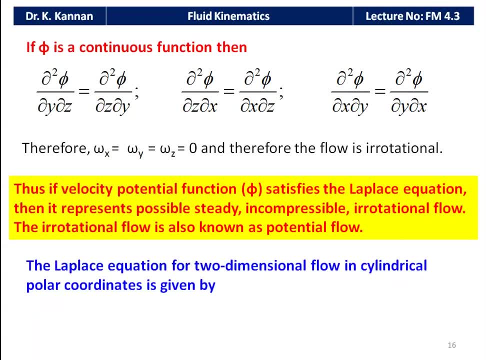 flow. The Laplace equation for two-dimensional flow in cylindrical polar coordinates is given by, so 1 by r dou phi by dou r plus 1 by dou square phi by dou, 1 by r dou phi by dou r plus dou square phi by dou r square plus 1 by r square dou square phi by dou theta square equal to 0. This is the Laplace equation for cylindrical, 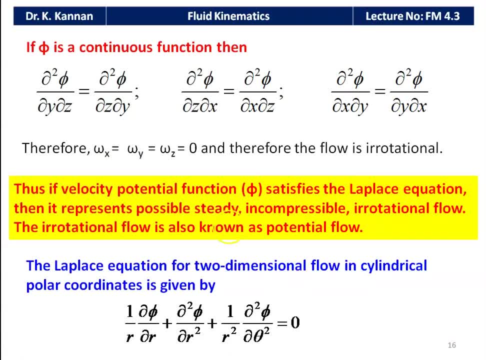 polar coordinate in two-dimensional form. And we stop here. So, the velocity, so we have to remember, we have to remember the velocity acceleration term, velocity vector, acceleration vector and we have to remember the vorticity and the condition for circulation flow and the condition for rotational flow. We have to define vorticity and circulation 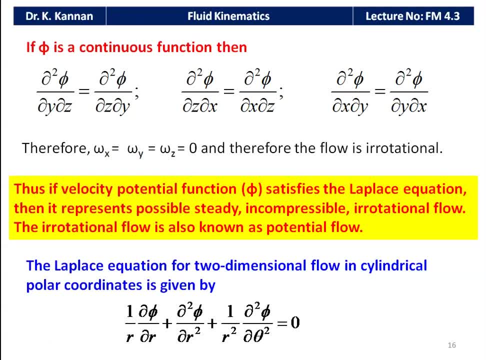 and we have to remember the velocity potential function and the conclusion for solving the problem. So, what is Laplace equation? What are the terms in Laplace equation? 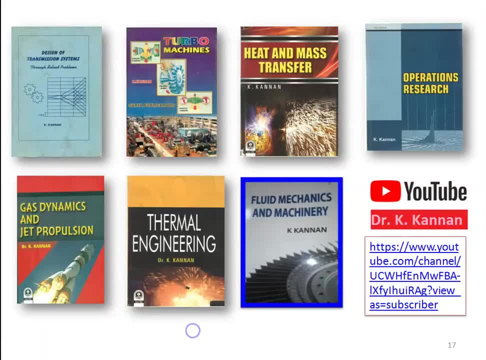 Everything you have to remember for solving the problem. So, we stop here. And these are all the books I published in the mechanical engineering subject, design of transmission system, 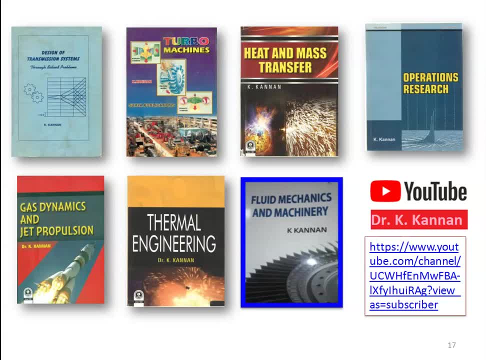 turbo machines, heat and mass transfer, operations research, gas dynamics and jet 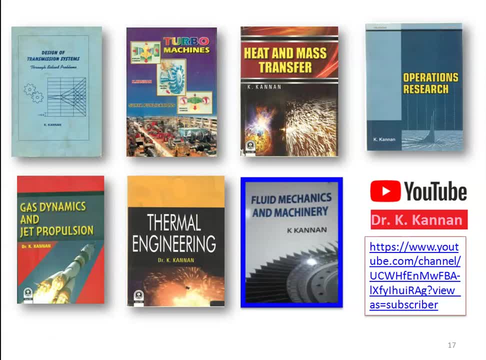 propulsion, thermal engineering, flint mechanics and machinery. And this book will be useful for additional information in this subject. And I have a YouTube channel where I upload the video lectures on this subject. You can refer to it. Use the videos for your better learning and to pass in the GATE examination. I am uploading the solution for GATE question papers also in the YouTube channel. You read it, use it and make a pass in the GATE examination. 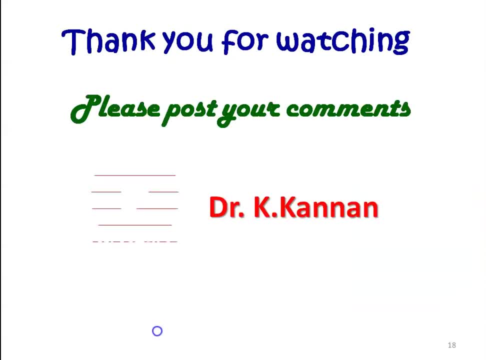 Thank you for watching. So, please post your comments on the comments box. So, you subscribe the channel so that you will get the updated videos. You can write to me to my mail id for any clarification. 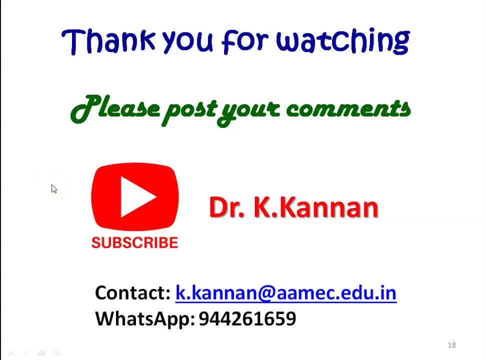 So, we will meet again in the next video with additional topics on the flint mechanics and machines.